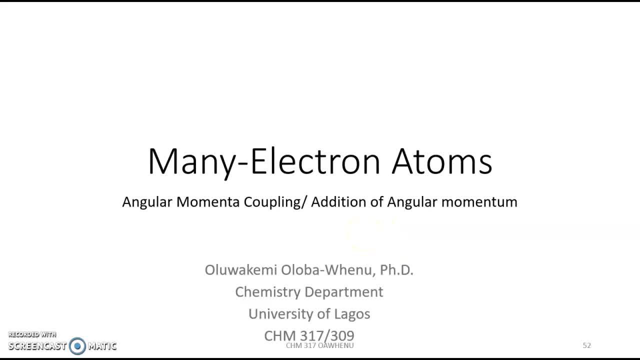 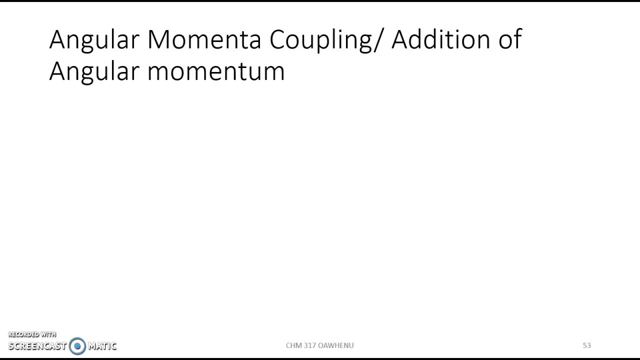 Welcome back to the lecture on many electron atoms for the Department of Chemistry University of Lagos. In this video we'll be talking about angular momentum coupling. Angular momentum coupling is the coupling between the several angular momenta in the electron. This is because, as a charged particle, 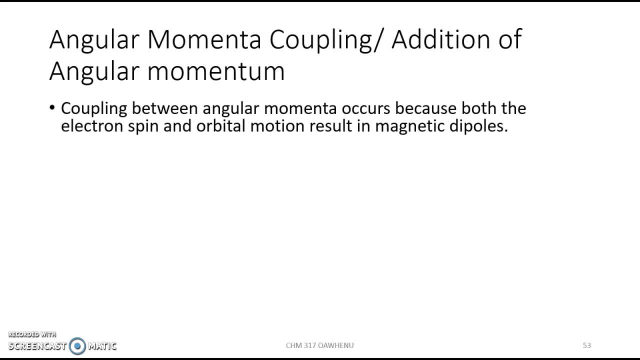 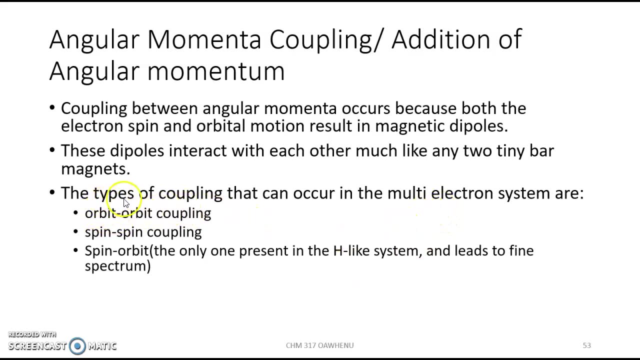 that's in motion. it behaves like little magnetic dipoles, and magnetic dipoles often interact with each other much like any two tiny bar magnets. The different types of coupling that can occur in a multi-electron system is a coupling between two orbital motions, a coupling between spin motions or a coupling between. 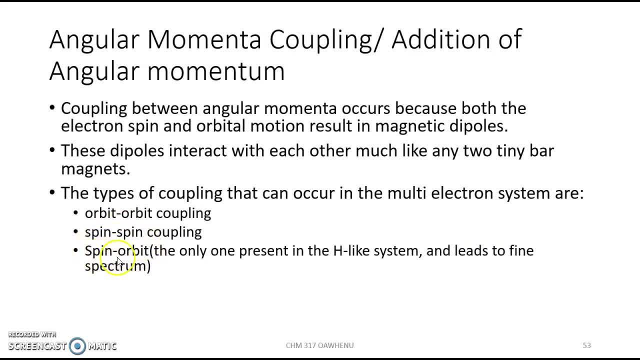 both of them, that's, the spin and orbit. The spin-orbit coupling is the only one present in an hydrogen like system and it leads to the fine spectrum, which is the splitting of atomic lines in the spectrum spectra of hydrogen. So let's look at each one by one. It's the fine spectrum, it's the. 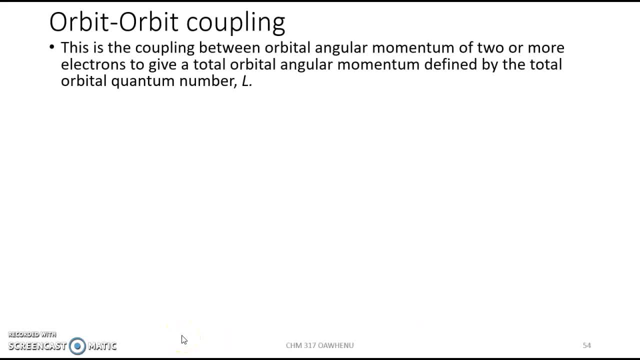 splitting of spectral lines. The orbit-orbit coupling is a coupling between several orbital angular momenta to give a resultant angular momentum L, capital letter L. So it's the sum of small letter L. So it goes from the coupling resulting numerical values from L1 plus L2 all the way to L1 minus L2, and they're. 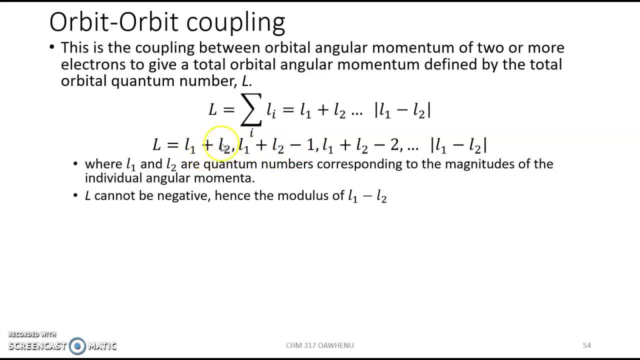 taken in integral steps. So the first one is L1 plus L2.. The second number is L1 plus L2 minus 1.. The second one is L1 plus L2 minus 2.. up until we get to L1 minus L2.. Now the modulus of 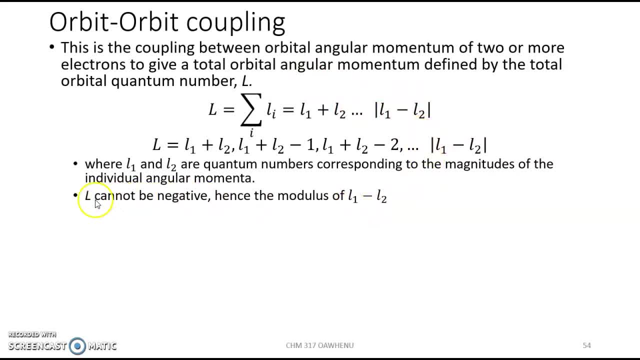 L1 minus L2 has been taken because L cannot be negative. L1 and L2 are the quouriants or quintal echtions of an integral. L1 and L2 are the quintuplets of various integrals and when you substitute these quadratives you will get a tak Justice line. 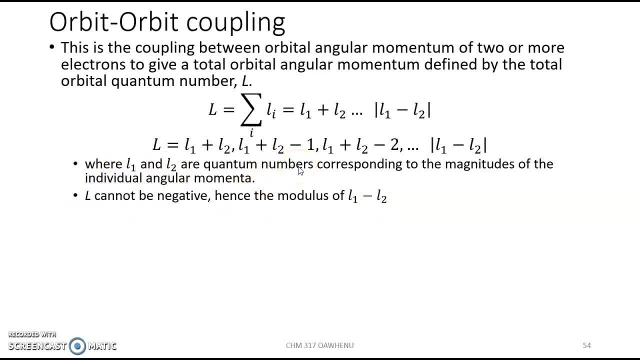 Also, you can't удивihadisq e n negativisq azmeaseksie skcat passionate or n? k Спасибоm. Thank you very much for your time. orbital quantum numbers of the corresponding electrons. Now, this is a. 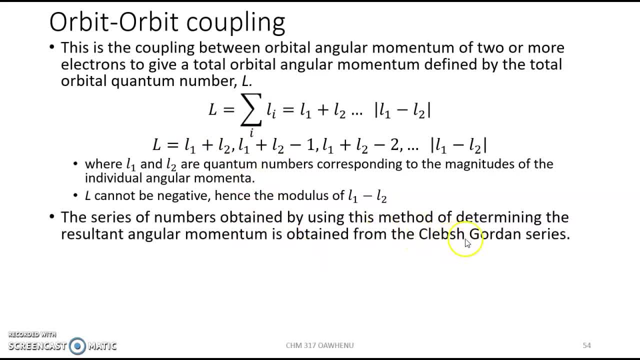 result from Klebsch-Gottard series and we're not going to go into the details of that. The minimum value corresponds to when the minimum value of L, the resultant L, corresponds to when the two orbital angular momentum are in their most opposite. 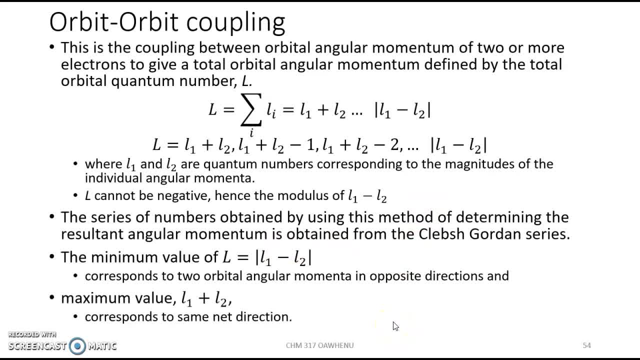 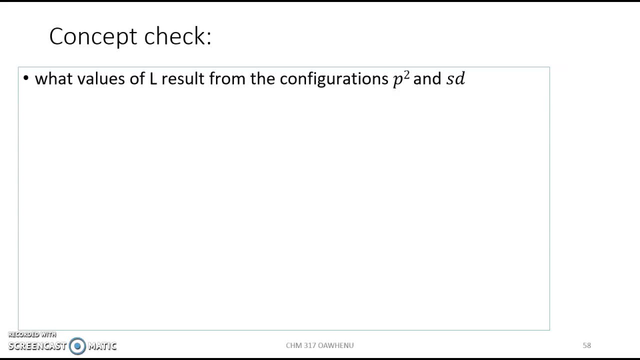 position and when they're in the same net direction, You have the maximum value of L. Then we have relative values, intermediate values in between. Let's take an example of this: What values of L as total result from these two companies? 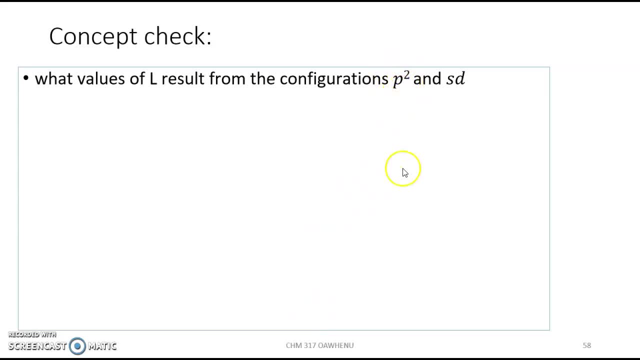 The two electrons in a P2 configuration, For that the first electron, L1, is 1 and the second electron, L1, is 2, here in the P-orbital, where L is 1.. Sorry, L2 is also 1,, not 2.. 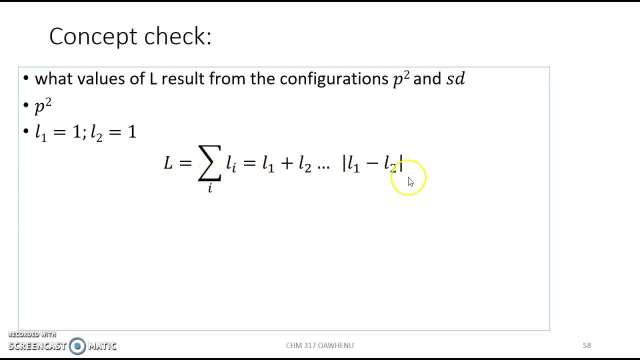 We have the formula L being given as that For both the P2 and P-orbital, two� values: L1 is 1 and L2 is 1, so 1 plus 1 all the way to 1 minus 1.. We have 1 plus 1 as 2 and 1 minus 1 as 0. We start taking. 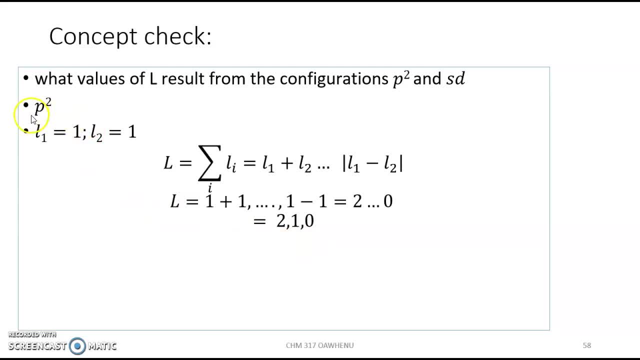 into into cross steps, We arrive at 2, 1, 0.. The L values that we can have from this configuration is 2, 1, 0.. configuration: The first: L is 0 and L2 is 2.. L is 0 for S, L2 is 2 for the D orbital. 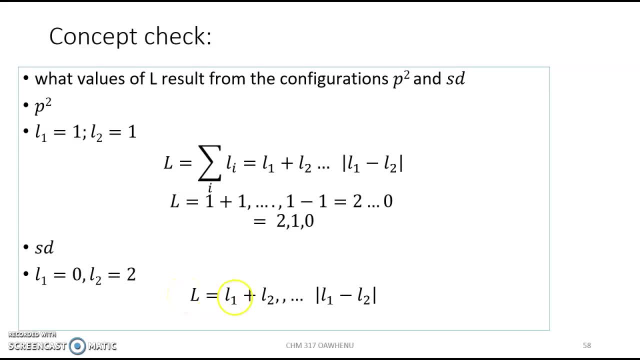 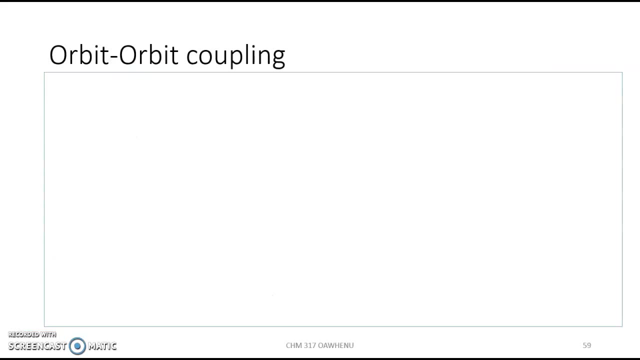 So again, our L1 goes from L1 plus L2 to L1 minus L2.. In this case it goes from 2 to 2, so we have only 2 as the value. It is possible that we are trying to couple more than two electrons. For example, nitrogen is Np if there are two. 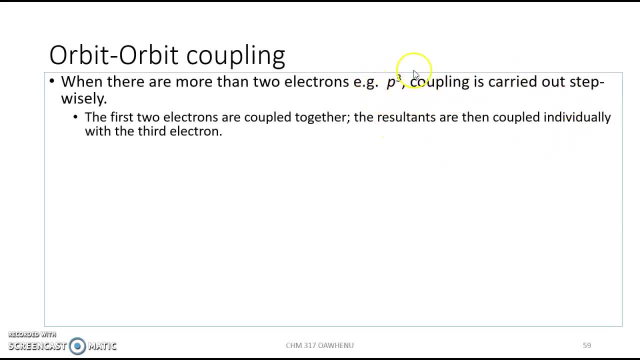 p if there are three. So how is the addition carried out? in this case? The first step is to couple two electrons together And then move on to the third electron. So in the p3 example, L1 is 1, L2 is 1, L3 is. 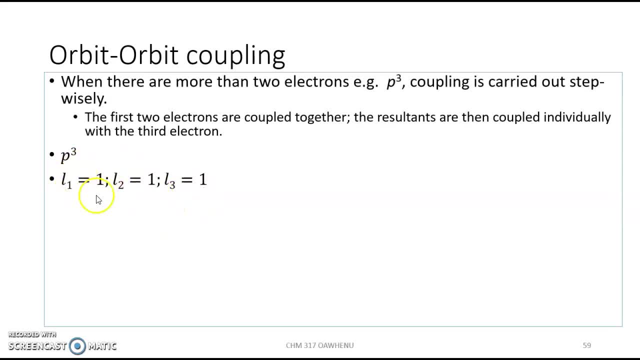 also 1.. So we take 2 and we call it L1, L2.. So that goes from 1 plus 1 to 1 minus 1.. So it's like the p2 example that we just did. So we have it as 2, 1, 0. 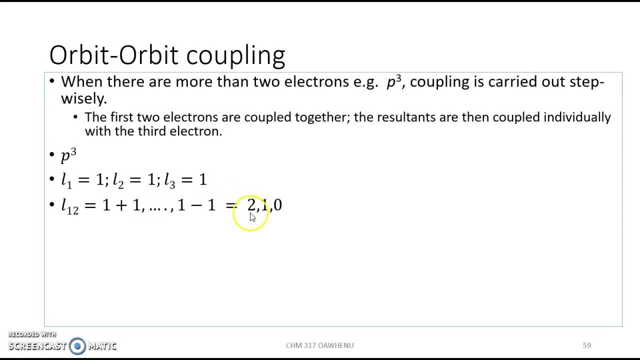 So that goes from 1 plus 1 to 1 minus 1.. So it's like the p2 example that we just did. So we have it as 2, 1, 0. So the next step is to couple whatever result we have here with a 1.. 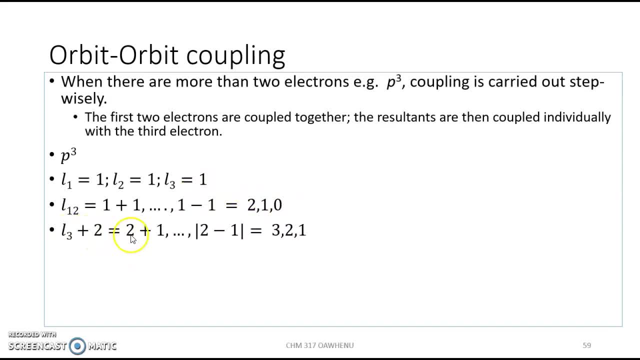 So taking 2, L3 plus 2, so we move from 2 plus 1 to 2 minus 1.. So plus 1 is 3, 2 minus 1 is 1.. In integral steps that gives 3 to 1.. So we take the next one, this one here: L3, 1 plus 1.. 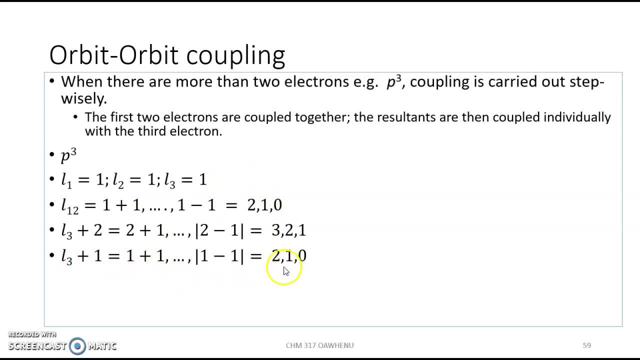 So it gives 1 plus 1 to 1 minus 1. That's 2, 1, 0.. And then, lastly, we have 1 plus 0. That gives us 1.. So the L values that we have are 3, 2, 1,, 2, 1, 0, and 1.. 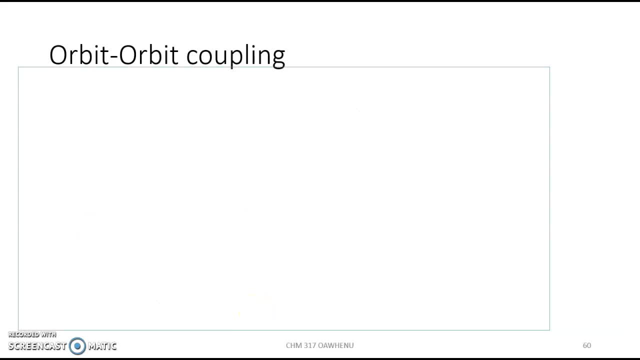 Those are the possible orientations that we can have. from that The states or terms For L, similar to the orbital quantum number, are also given the capital letters for L. So in the case of the p2, where we have the resultant L values being 2,, 1,, 0,, 2,, then we have the capital D states representing 2,. 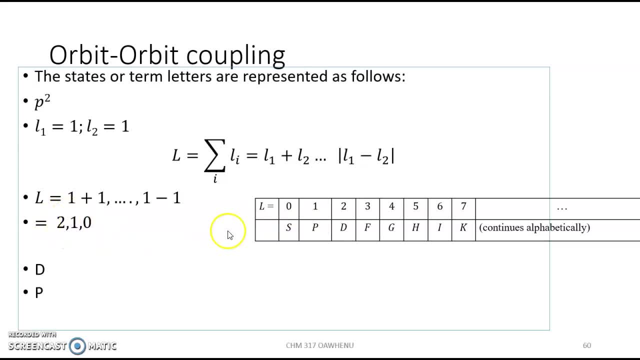 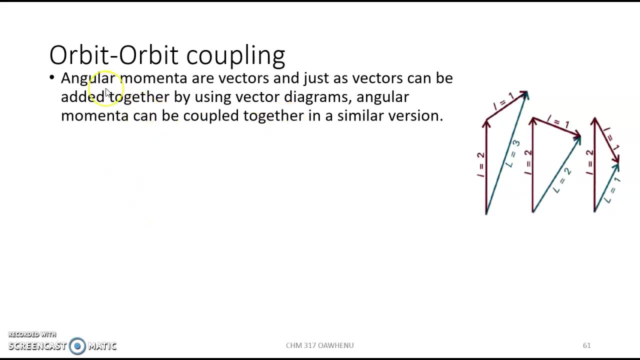 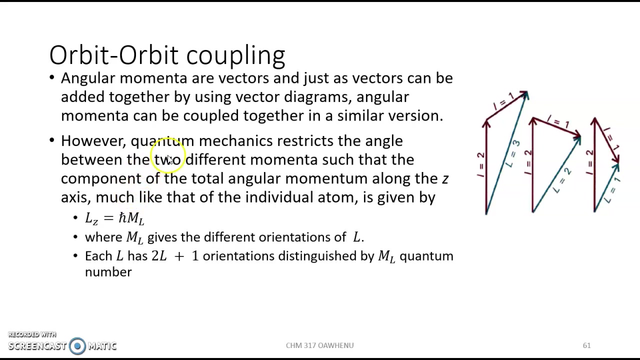 the capital P states for 1, and the capital S states for 0.. One other thing before we move on to the spin is that angular momentum are vectors, and vectors can be added together. However, quantum mechanics restricts the angle between the two different momenta such that for each L 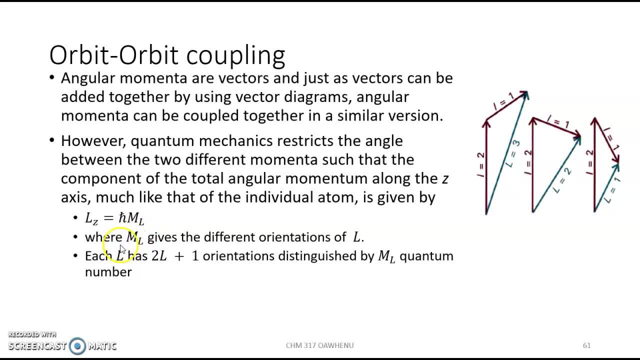 we have the Lz. So, for example, we have a component which is related to our M sub L. This is similar to the M sub L magnetic quantum number of the hydrogen atom. So each L has associated with it M L values which goes from 0, sorry, from minus L- through 0 to L in integral. 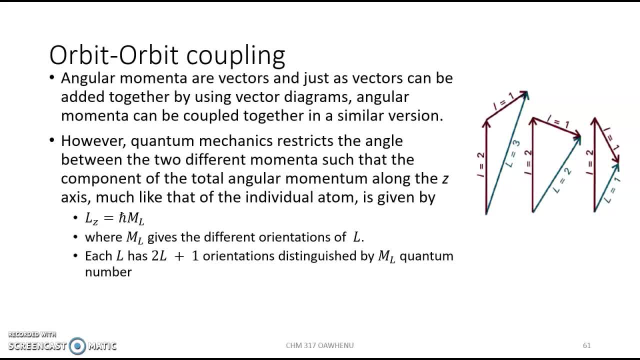 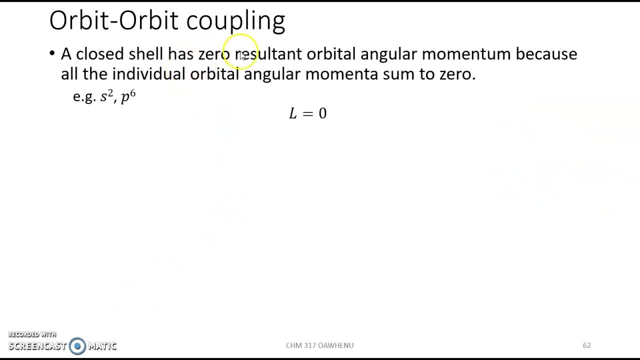 Steps again, much like the value of the angular momentum for the orbital angular momentum and the magnitude of each total angular momentum is also given as that A closed shell. one other thing is that a closed shell always has zero angular momentum. 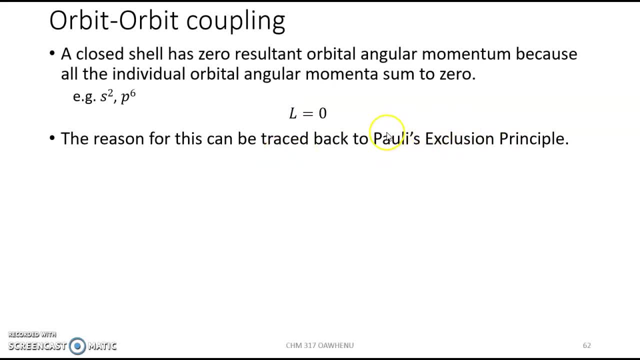 And the reason is because of Pauli's Exclusion Principle. So if we are given electronic configuration of S2, L can only be 0.. P6, L can be 0.. If we are given D10, L can only be 0.. And at the other restriction point, P6, L can only be 0.. And at the other restriction point, P6, L can only be 0.. And at the other restriction point, P6, L can only be 0.. 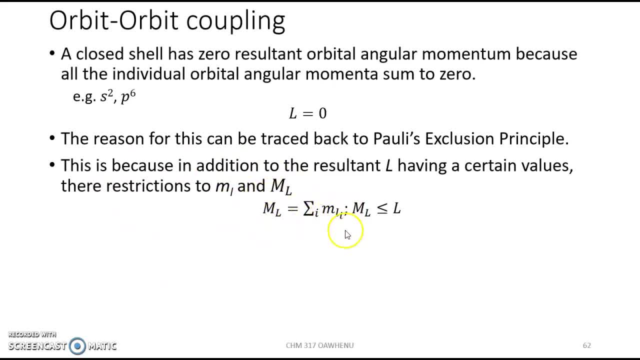 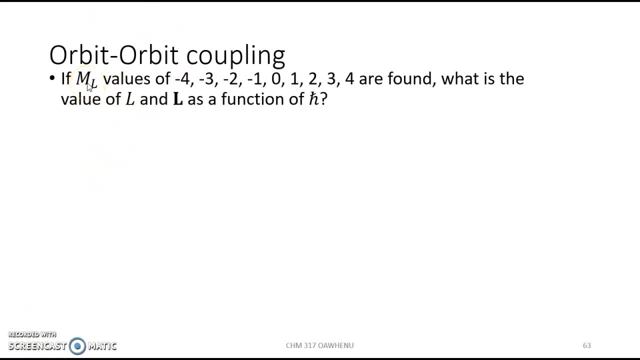 The final restriction is that M L, the sum of M L I, is equal to capital ML. So the question is: There's a question: If ML values of minus 4, minus 3, minus 2, minus 1 are observed, what is the value of L?